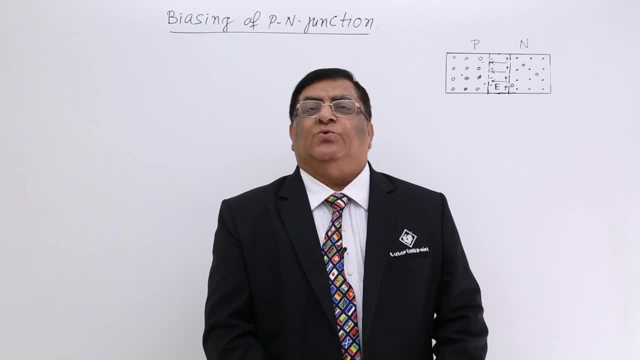 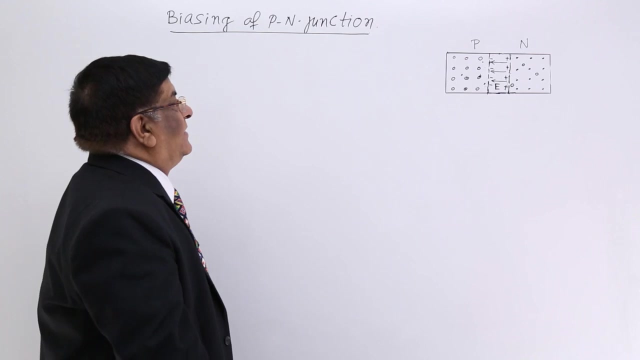 across a semiconductor. Now there can be 2 methods how we can apply EMF across, or potential difference across a semiconductor. These 2 methods are known as methods of biasing, giving potential difference across semiconductor. So one is known as forward biasing and one 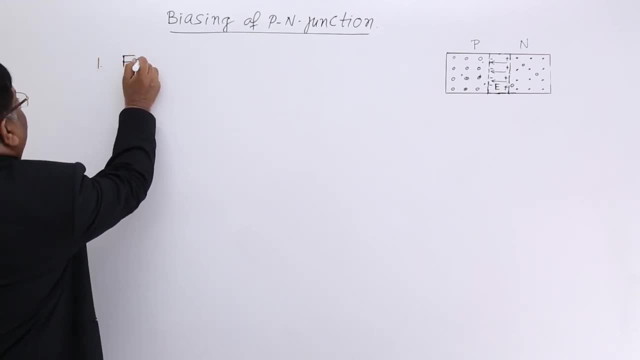 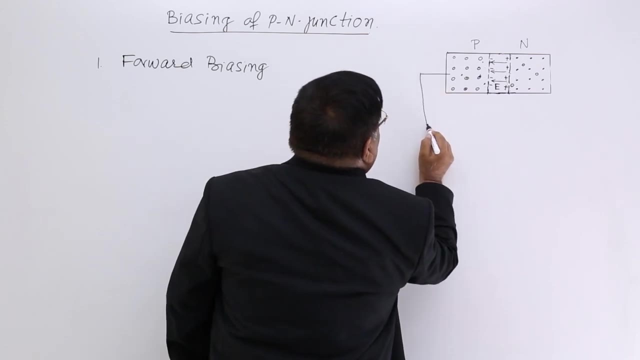 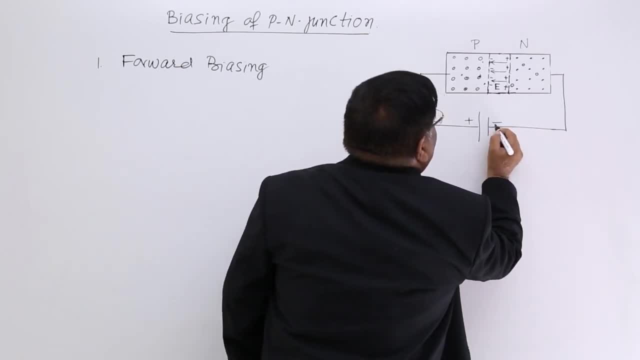 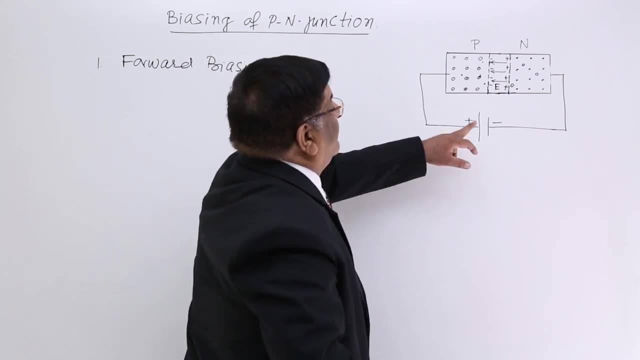 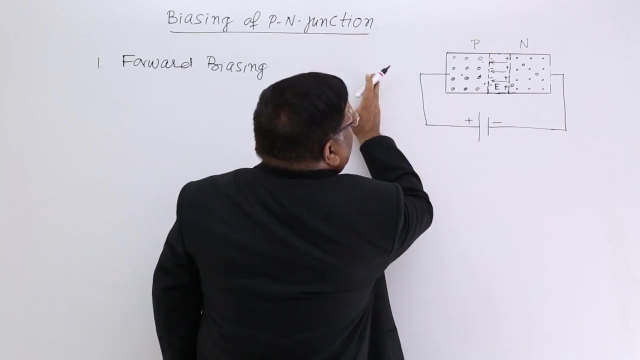 with negative side of the cell, Minus with n and plus with p. Now what effect does it have? When we connect it, switch it on. This is positive. So this press all these positive side of the cell repel. So there is a pressure from here on positive and there is a pressure. 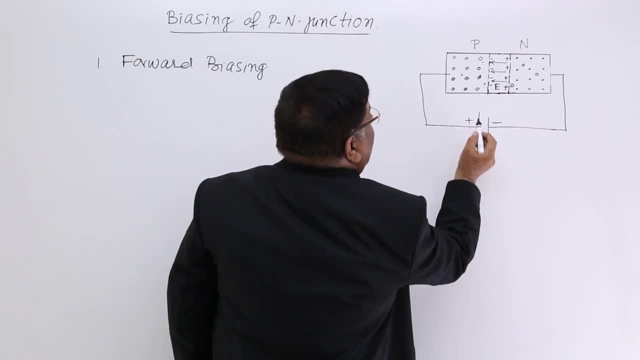 from here on negative. As a result of that, we see this layer has gone here and this layer goes here, So we get the new layer like this: and now they are closed, So this depletion layer shrink. So in forward biasing, 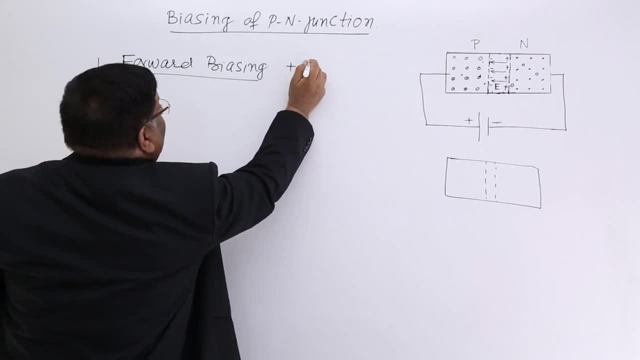 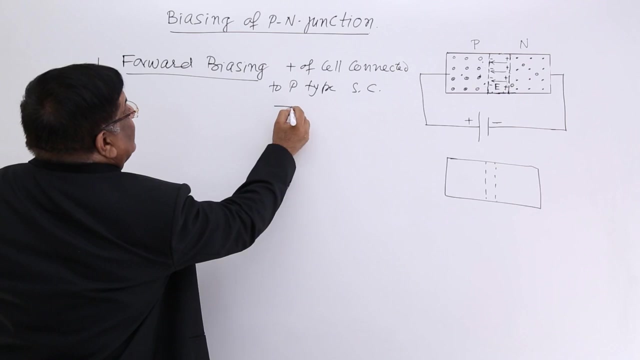 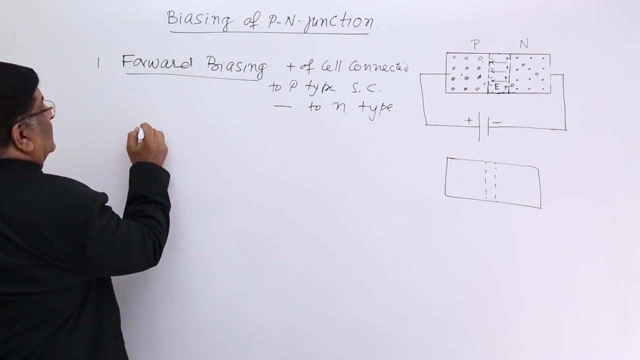 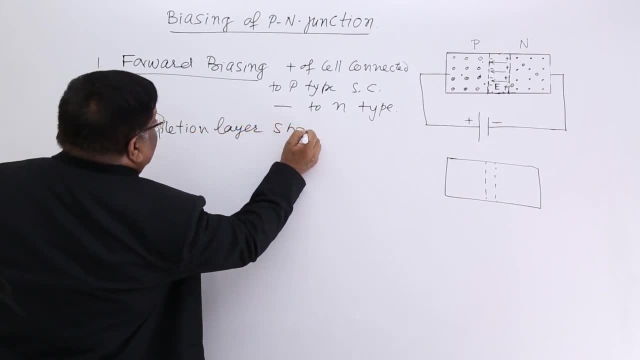 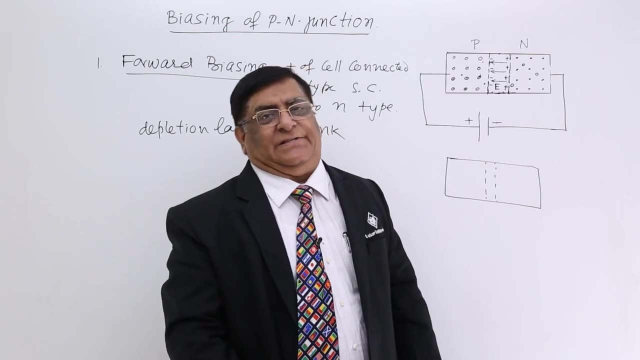 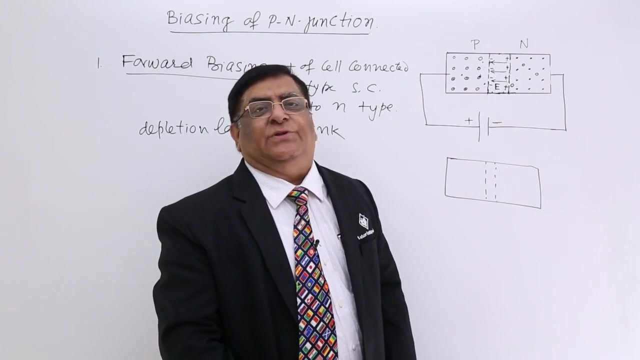 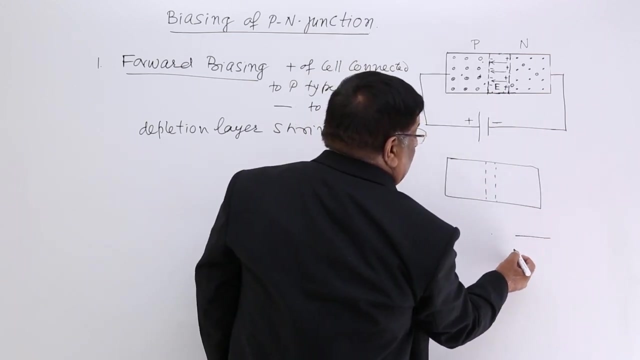 Depletion layer, Depletion layer shrink. And if depletion layer shrink you may say the resistance is decreasing. More than depletion layer study, it is very important to study what happens to the potential barrier. Here there was a potential barrier, high potential and barrier. 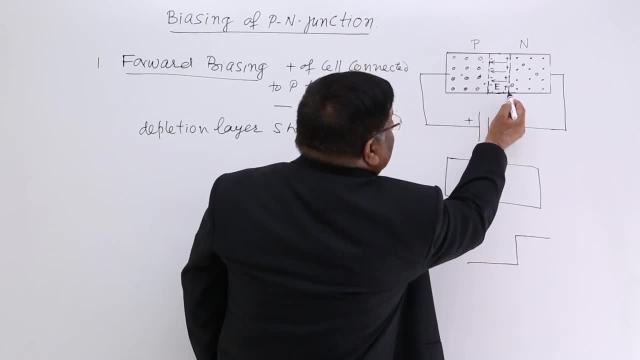 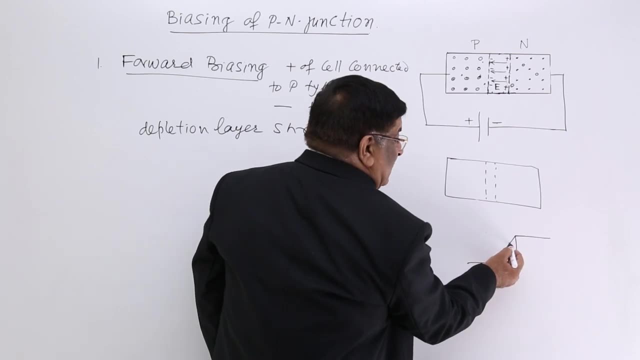 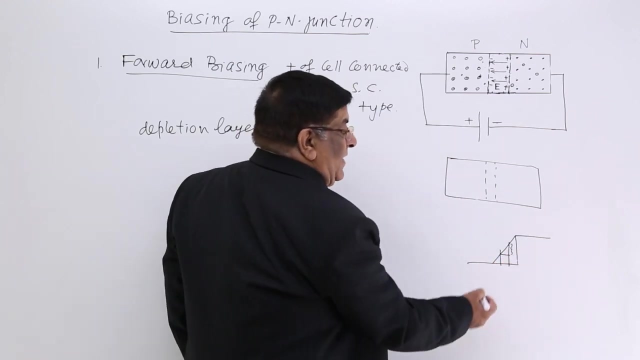 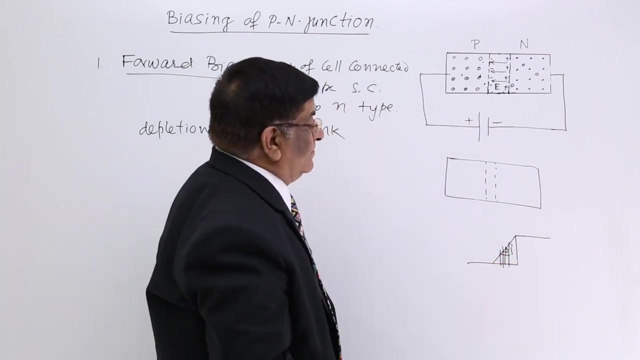 and low potential. This was the discharge. Discharge, this was the distance and this was the distance. now this is decreased. when this is decreased, it has come to this level now. how much is the potential barrier? this much. if it is decreased further, the potential barrier will be only this much. 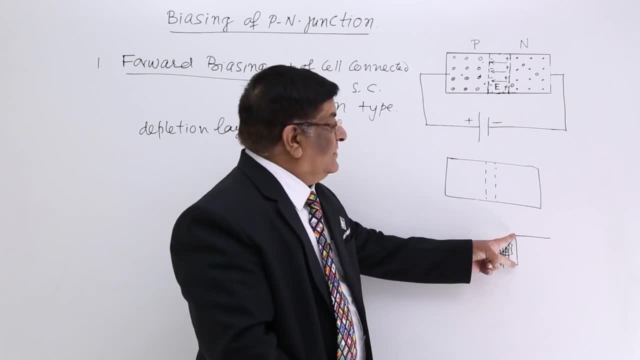 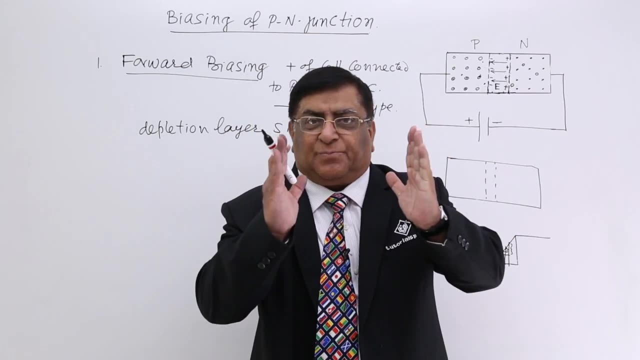 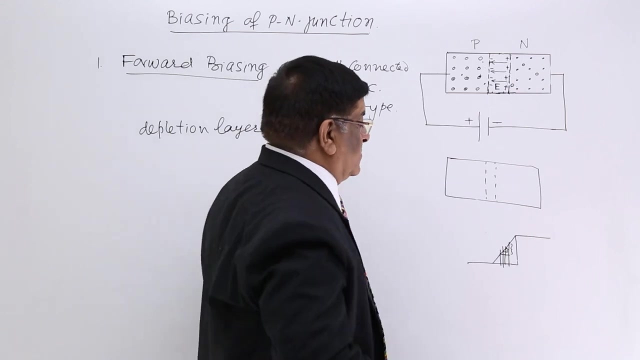 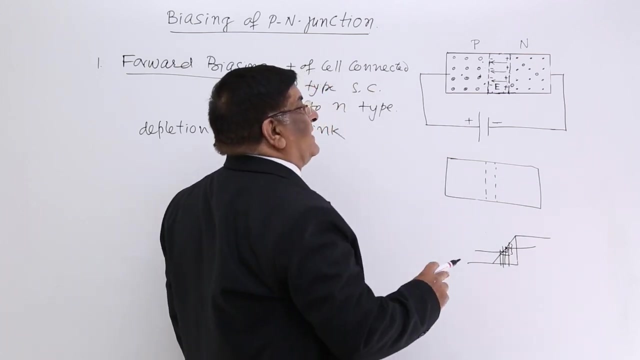 what is the unit of potential voltage? so this volt, 5 volt, 3 volt, 2 volt, 1 volt. so when depletion layer keep on shrinking, the potential barrier gets lower. so this is what's happening with the potential barrier. now you can understand it the other way. what is the direction of potential here? 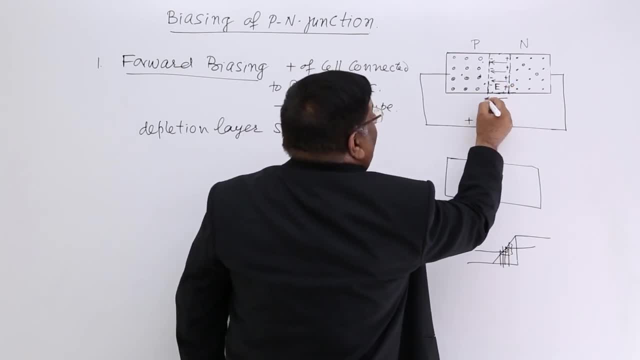 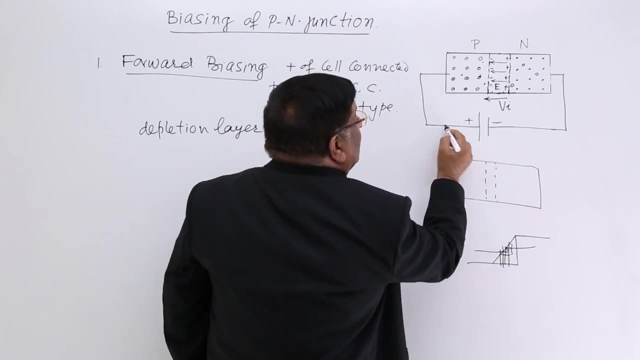 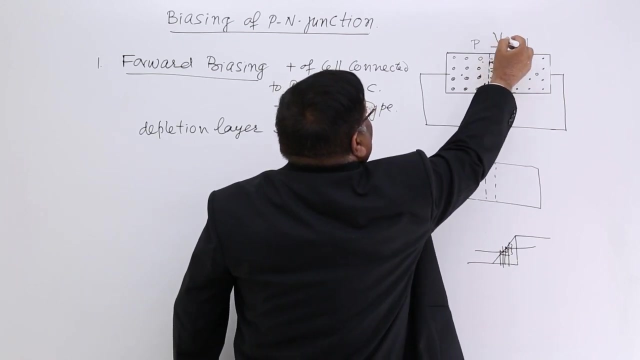 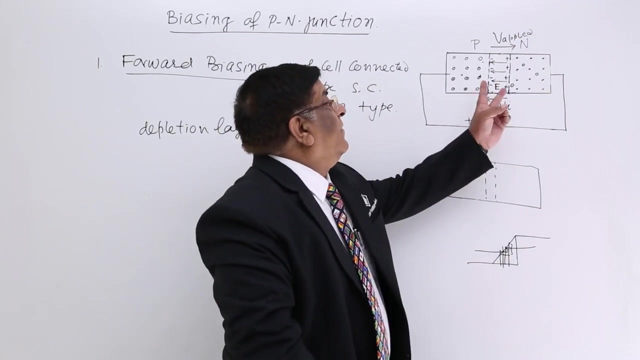 plus to minus. this is the direction of this. let's call it induced potential. we induced this potential, we apply. here is plus, here is minus. so this is the direction of: we applied and you see the directions are opposite. then what will be the potential difference here? answer: the potential difference will be algebraic sum of the. 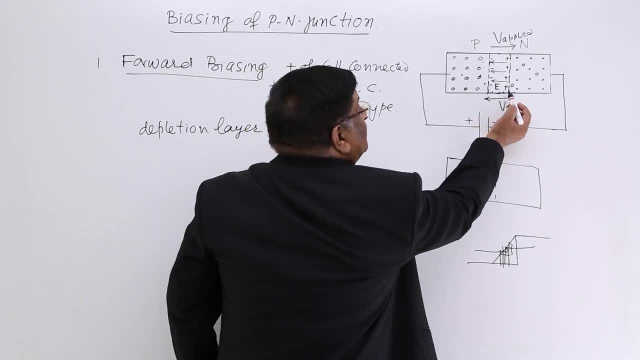 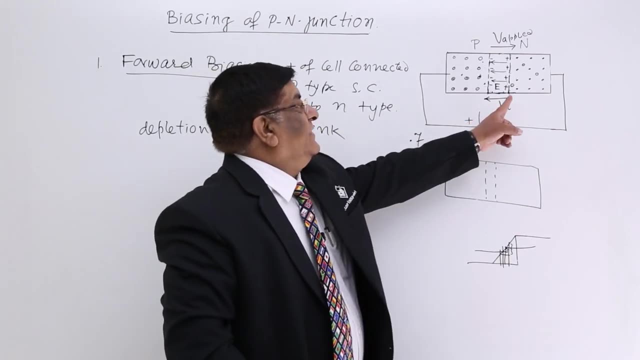 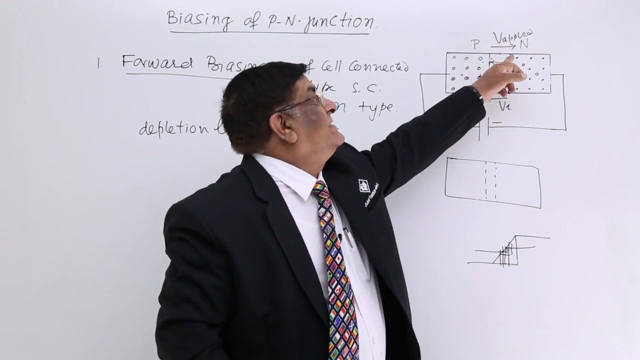 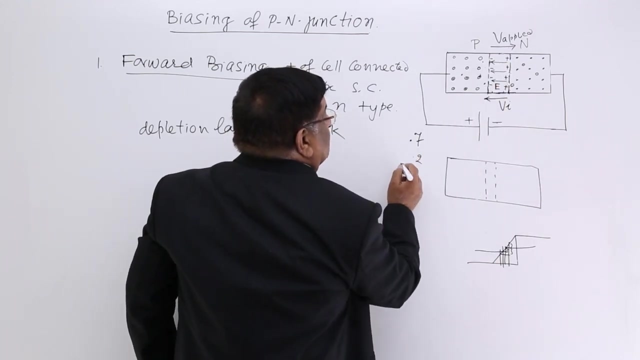 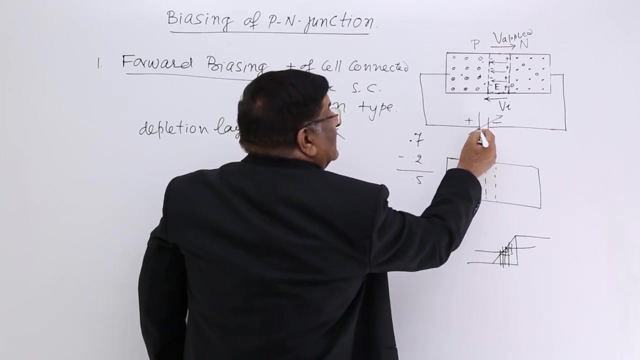 two sum. now, if this potential difference is equal to 0.7, this okay, then this we are applying here. this is say, 0.2 in this direction, 0.2. so what will be this? now, 0.5, suppose we increase this and make it 0.4, then what? it will be? 0.3 in this direction, if it is 0.3 in this. 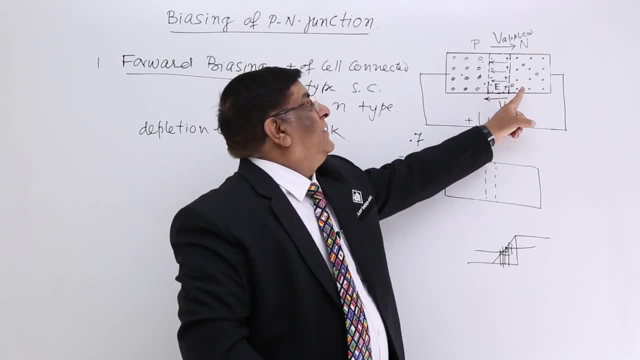 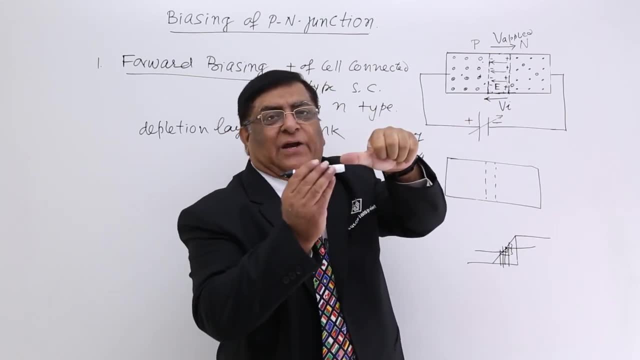 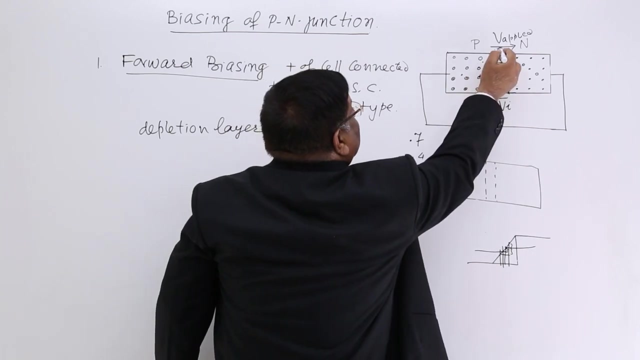 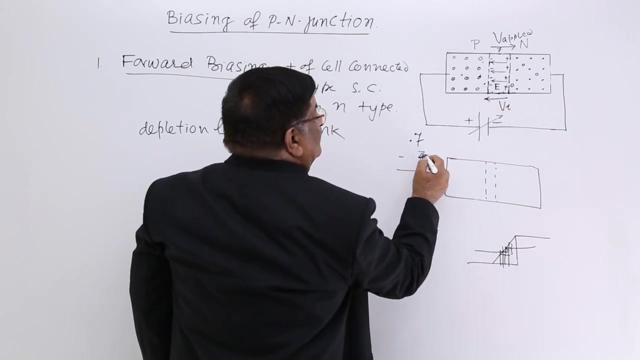 direction. still, this positive cannot go here, this negative cannot go here, because the resultant voltage is in this direction and electron cannot go. this will oppose. now we increase it further and make it 0.2.. 0.7. if we make this 0.7, this is also 0.7. now how much is the resultant? 0? that means 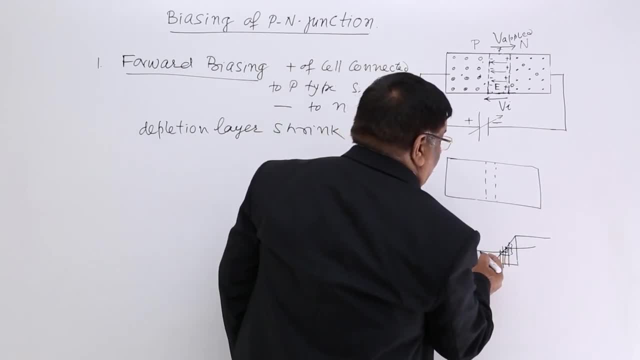 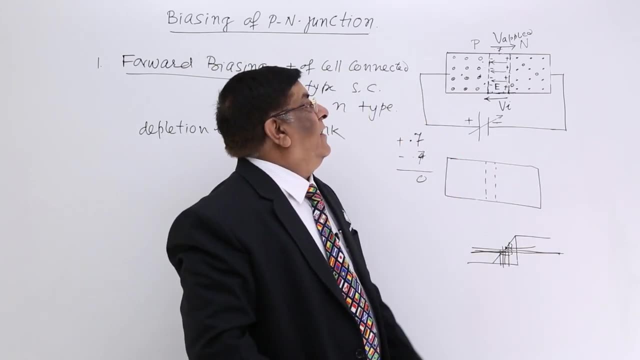 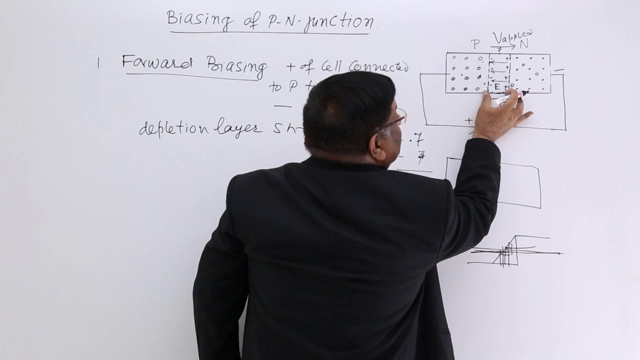 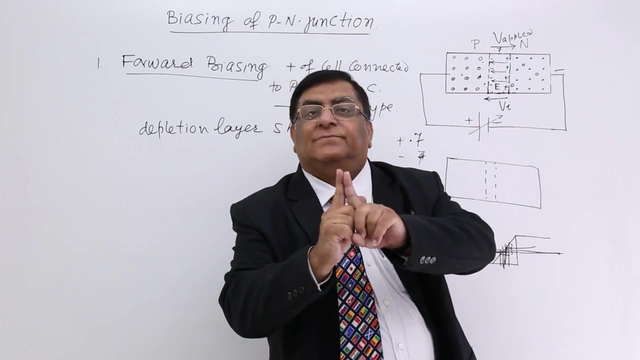 there is no potential barrier and both the potential have become same level, same potential. now, if there is same potential, all these electrons they jump. Now there is, This layer has shrunk, shrunk, shrunk and there is no layer. the layer has collapsed. the potential 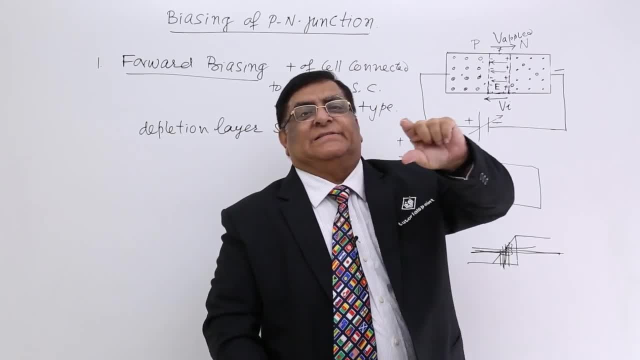 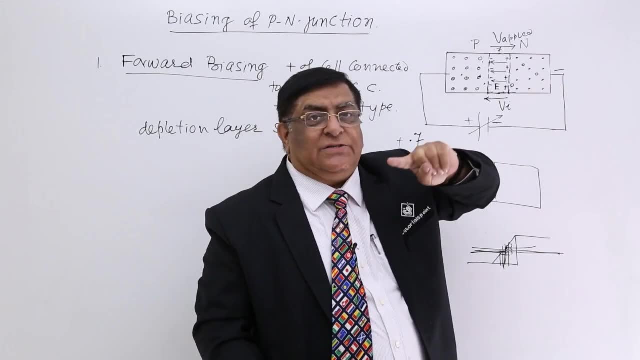 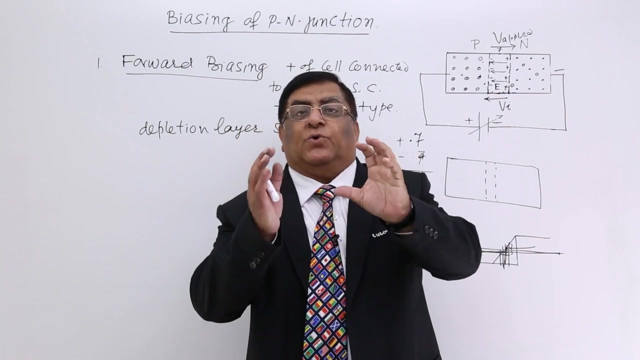 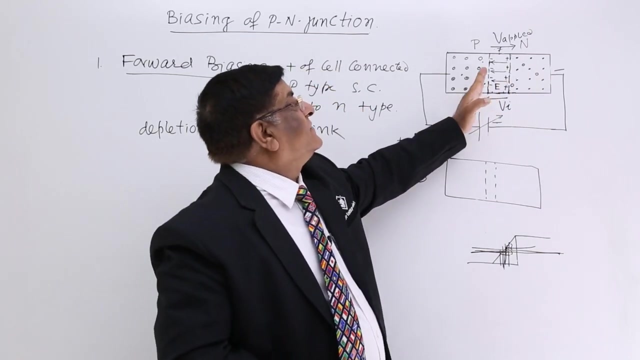 barrier has collapsed. now it has become a very simple semiconductor which has got a large number of charge carriers, because the number of charge carriers are very large and there is no depletion layer in between 0.3.. 0.4.. it potential, which we call potential barrier, to cross it, so all these electrons can run. 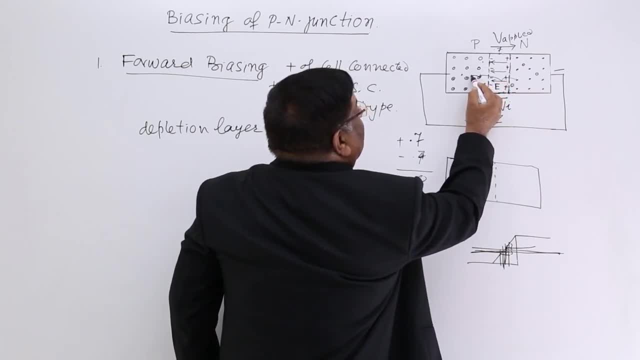 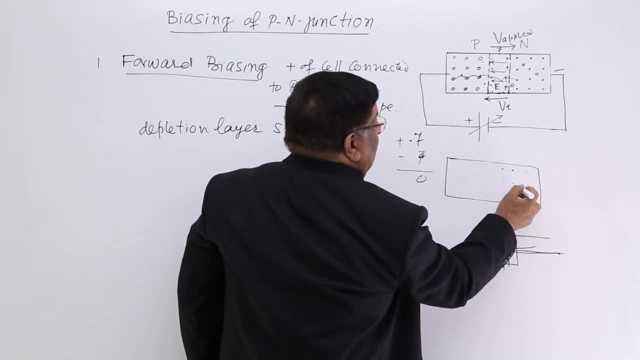 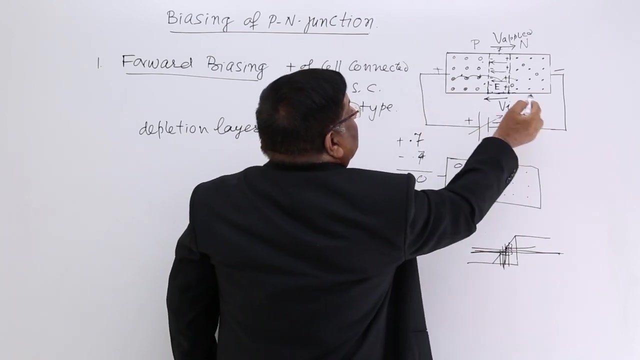 freely, so they run freely and come here, here, here this depletion layer is gone and now it has got majority of electron. this has got majority of holes, so it is very convenient for them to jump like this. and this side is what plus, this is minus, so this electron jump. 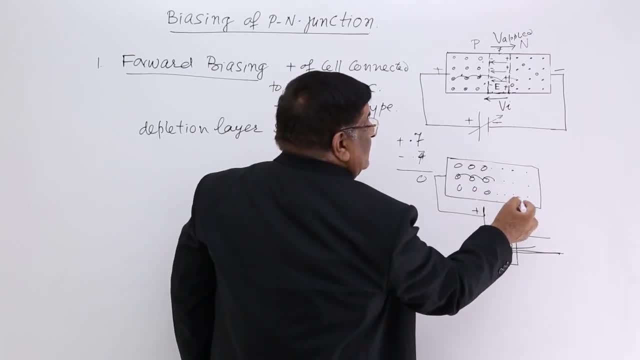 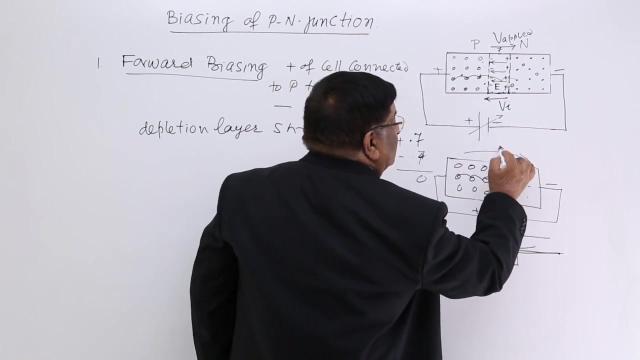 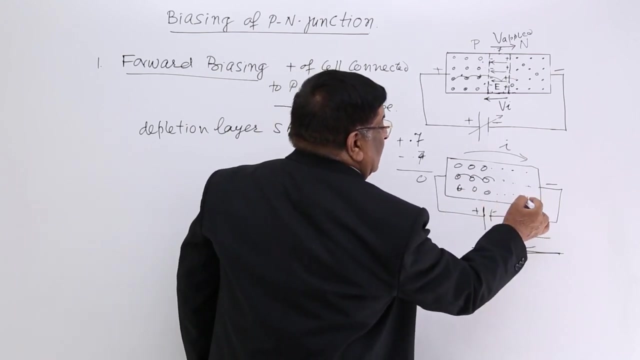 comes to plus, go to battery, then this electron come, this come, this come and this electron will come from here. minus, so electron go like this, so current flow like this opposite to the direction of electron. So we can say these positive are moving in this direction, electrons are moving in this. 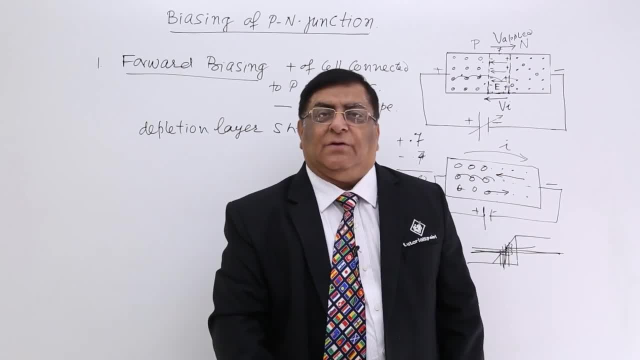 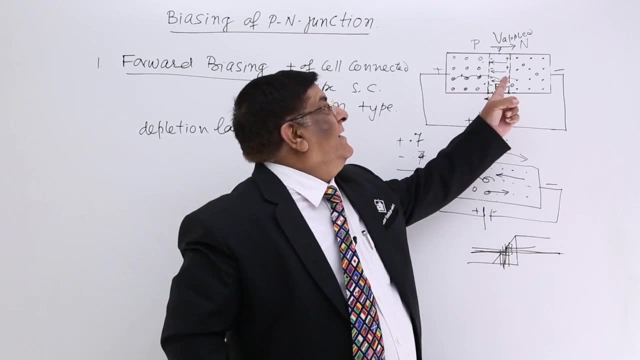 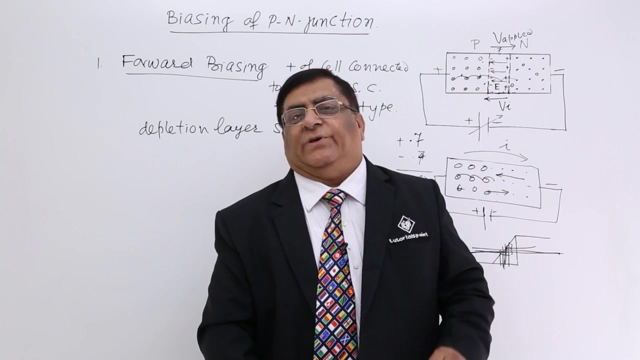 direction and the current start flowing. there is no girth of charges because there are number of charge. we have created in n type and p type. all those charge carriers are now in action and there is a good current flowing in that and it has become a conductor because 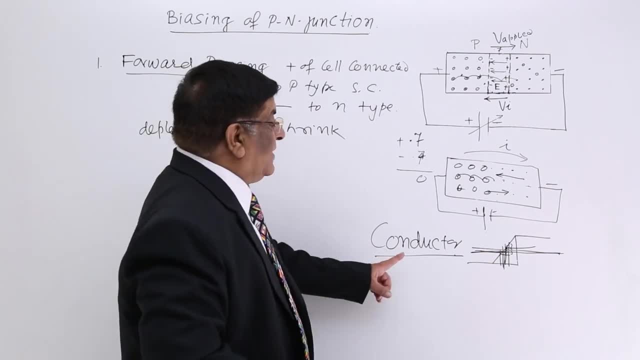 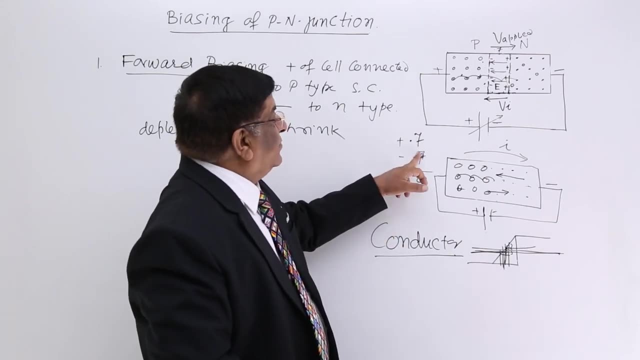 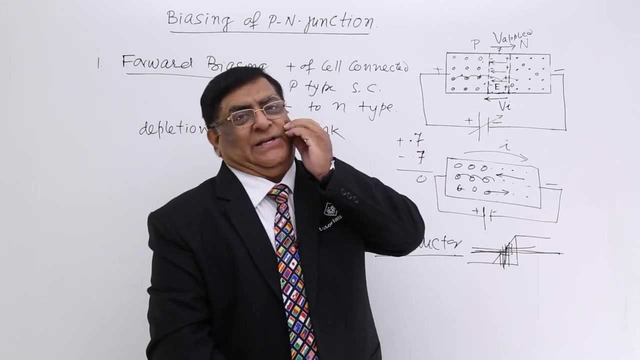 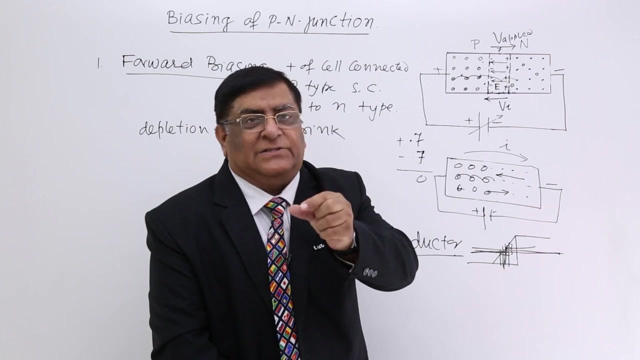 current is flowing when it has become a conductor, when the potential difference applied by us has become equal to the induced potential difference or which has become equal to the barrier potential. So when applied potential cross the barrier potential, then only depletion layer is destroyed and then only this mixing start and they start flowing.